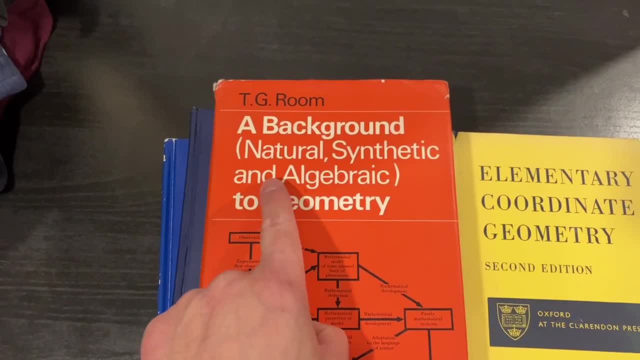 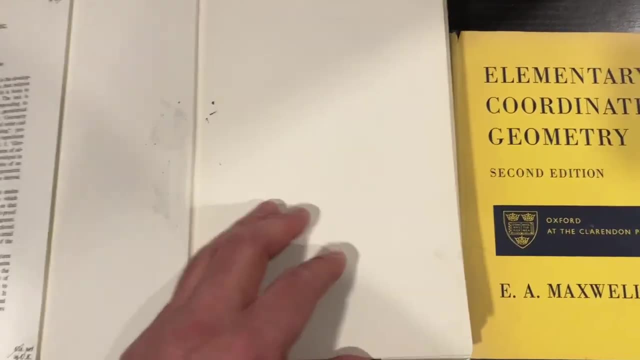 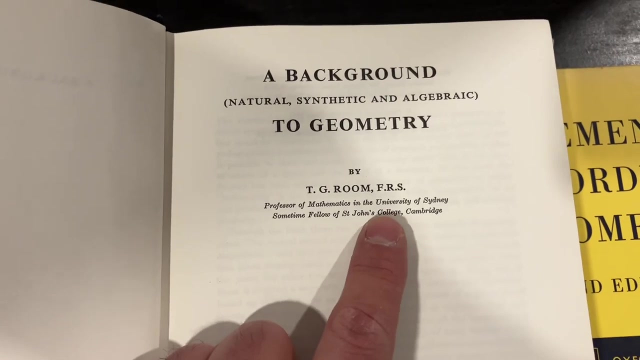 all of these, I have here a background on natural, synthetic and algebraic geometry. Well, I was checking this text and it's very strange: They don't use numbers. It's by Ruhm, actually Right from in Australia. He's from Australia University of Sydney. 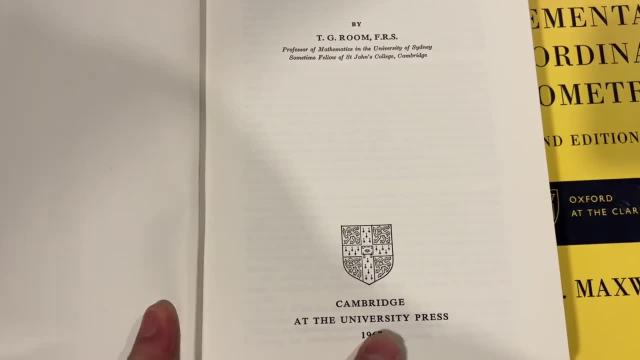 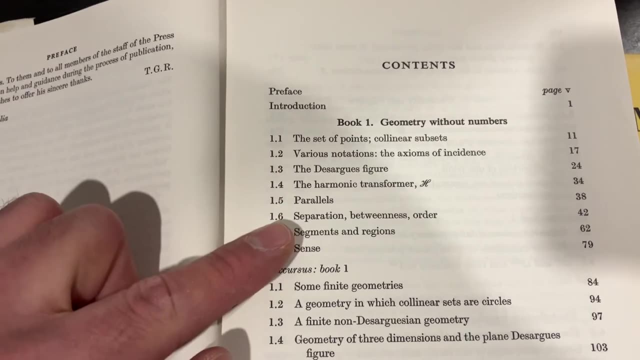 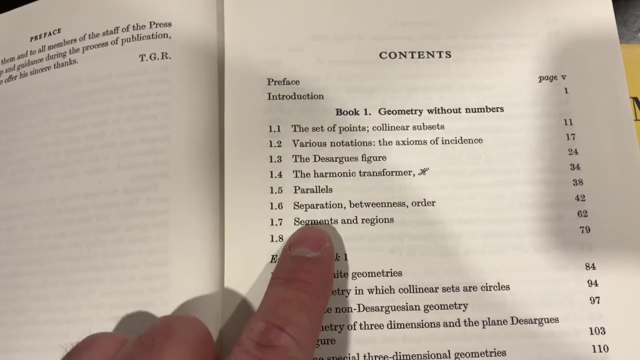 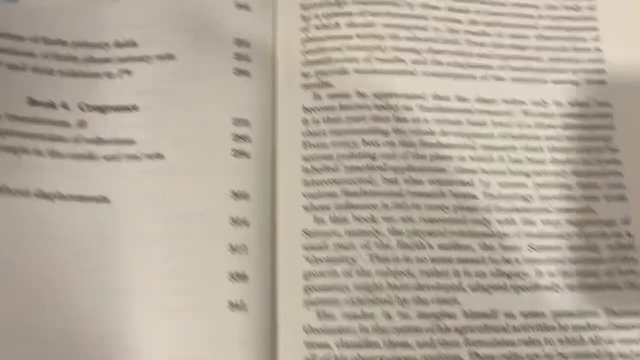 And the edition is by Cambridge at the University Press 1967.. Geometry without numbers, It's just, you know, abstract definitions on, you know parallels, a what's, you know a set of points, separation, axioms and stuff like that. Geometry and counting here, And then we have geometry and algebra. 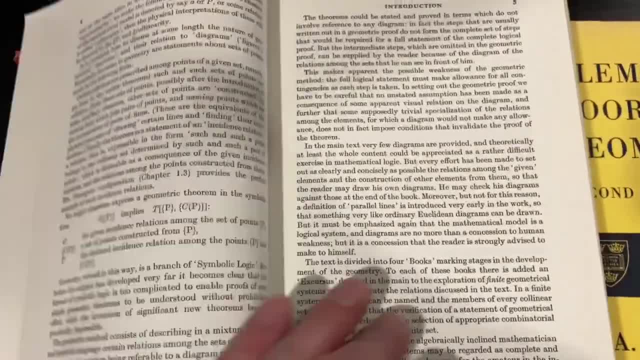 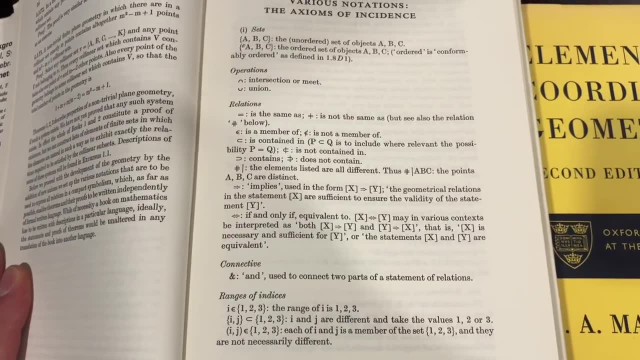 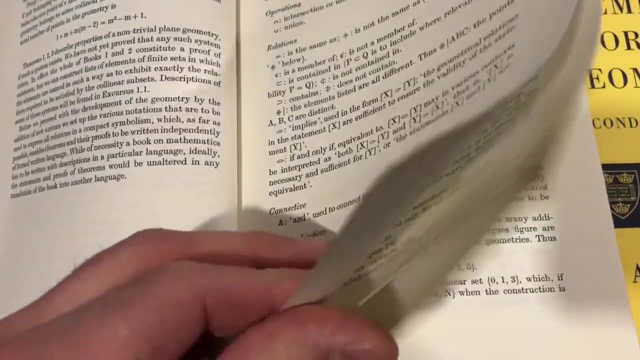 Congruence as well. It's a very strange textbook, See. it's, like you know, some of the older textbooks on logics, mathematical logics. they don't use numbers at all. I think I have a few. I'm going to talk about those in a future video. The next one is by 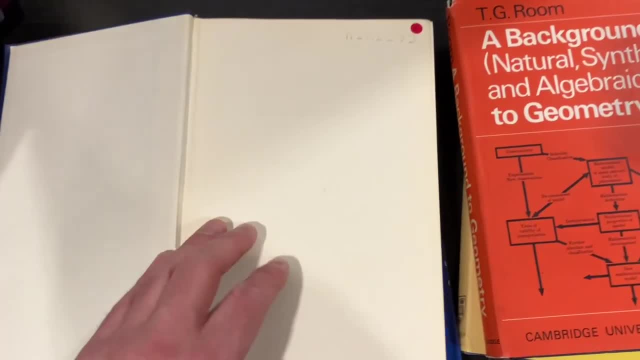 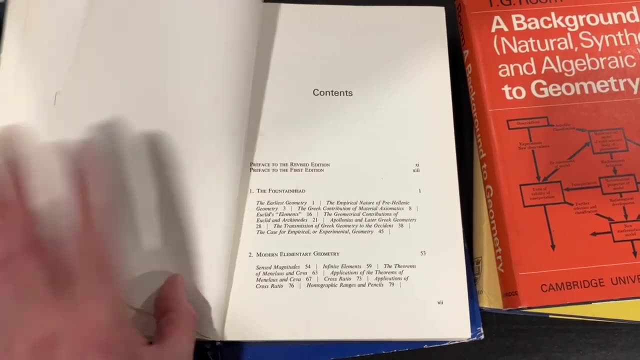 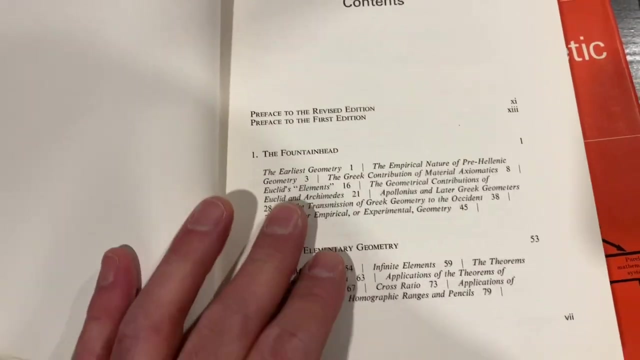 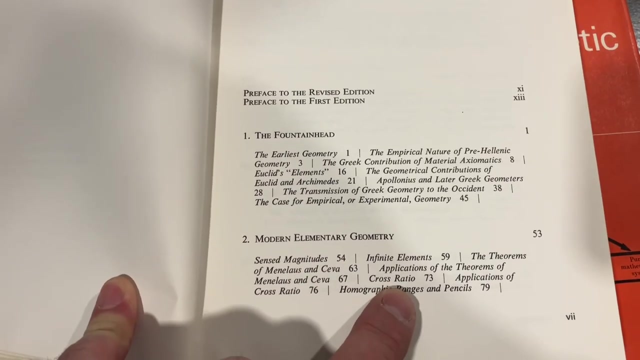 Howard Eaves A survey on geometry, Survey of geometry, And this is a very good textbook. actually, This textbook is on Euclidean geometry, So let's quickly go over the contents: Modern elementary geometry- down here. Cross ratio- down there. Homographic ranges and pencils. 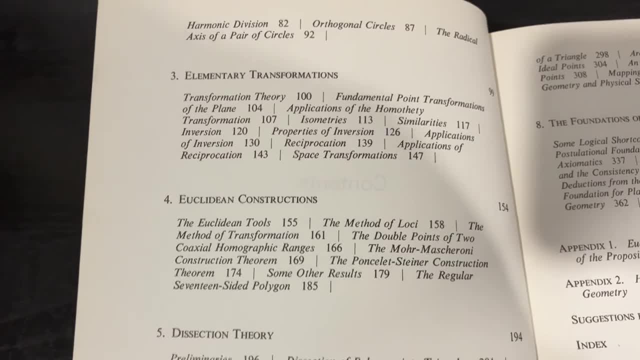 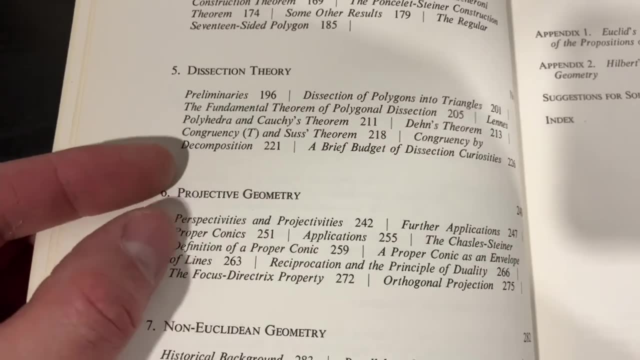 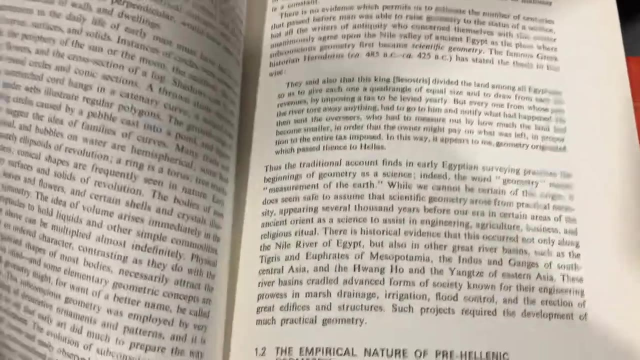 Uh, Euclidean constructions, Elementary transformations, And then look, Projective geometry. This is super interesting, Super, super interesting. Non-Euclidean geometry, The foundations of geometry, down here. So it's it's a very, very nice textbook, I believe. 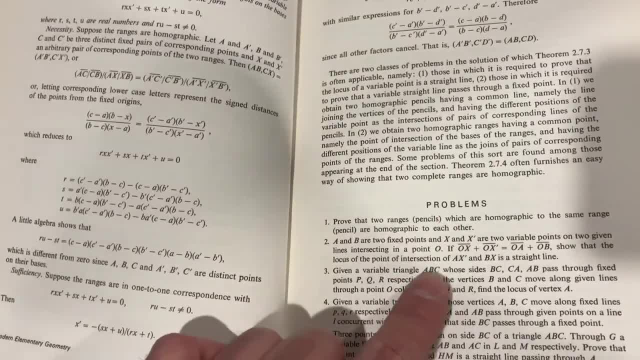 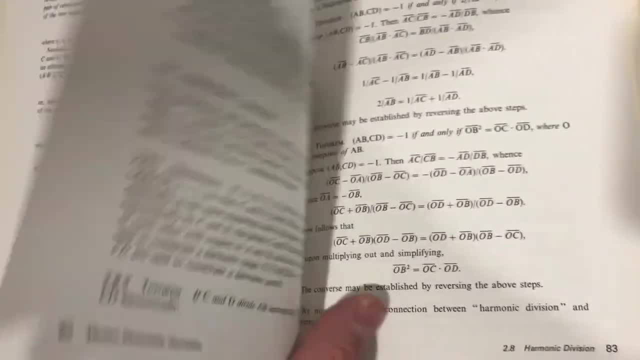 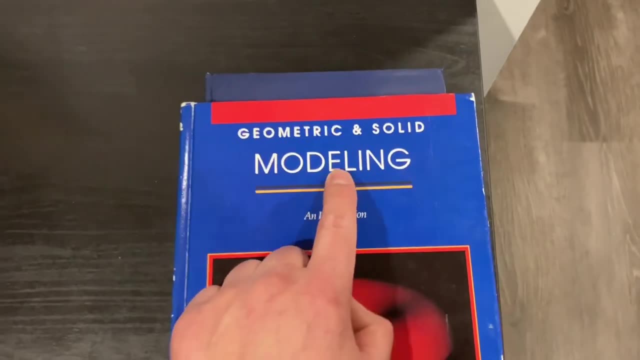 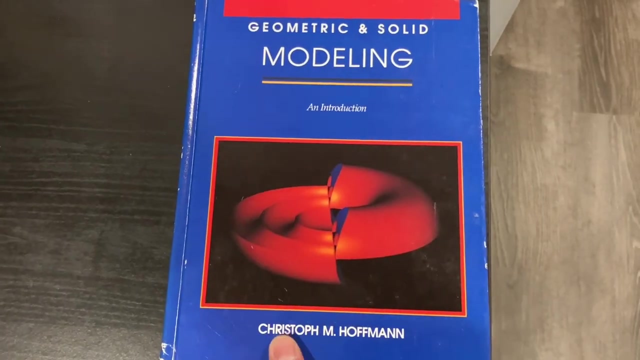 there's a bunch of problems, Yes, scattered around here and there. Harmonic division: It's a very nice textbook on Euclidean geometry. You can check it out, guys. The use of geometry in modeling, So geometric and solid modeling, actually by Hoffman. Look at this. 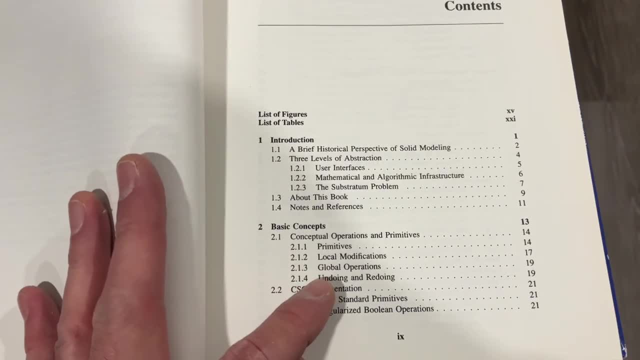 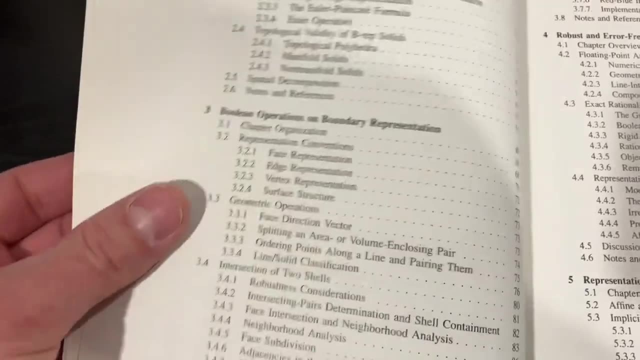 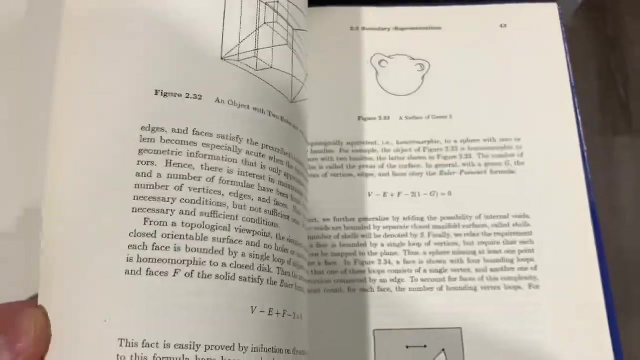 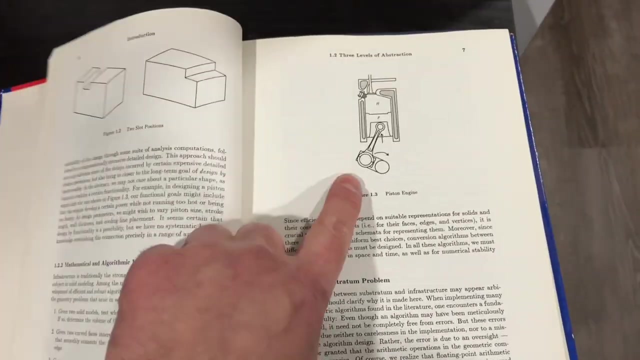 Three levels of abstraction, Basic concepts down here. This is a kind of strange textbook actually Boolean operations on boundary representation. So I think this is not immediately related to you know, Euclidean geometry. It's geared toward um applications of you know, planar Euclidean geometry. 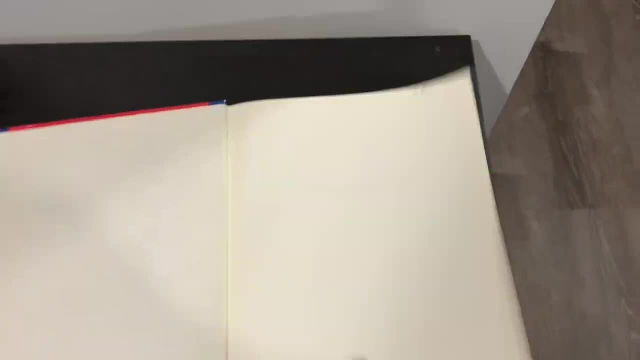 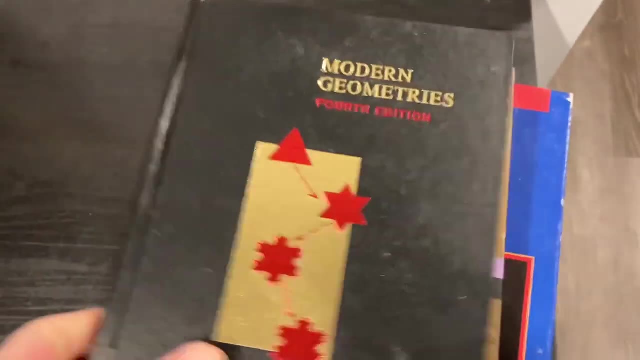 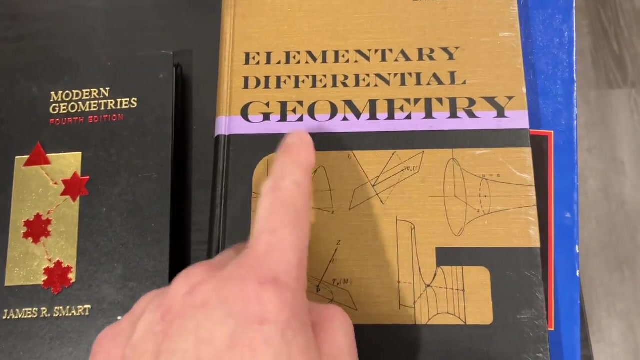 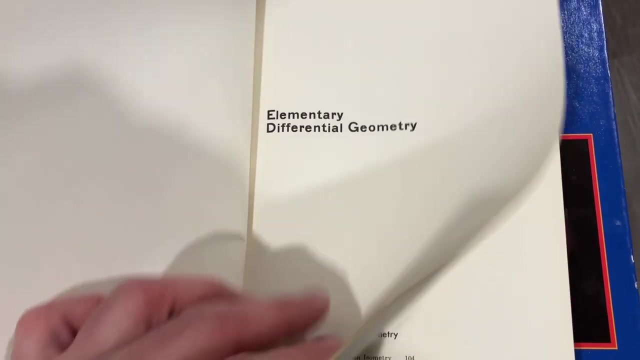 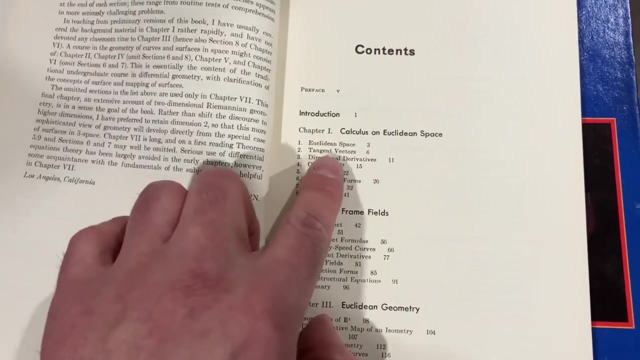 Modeling and stuff like that. And let me quickly go over two beautiful, beautiful actually textbooks. And the first one is: this is an interesting one, It's a sort of introduction to actually differential geometry. But this textbook treats, you know, the dimension 3ks, Elementary differential geometry by Barrett O'Neill, down there Calculus on Euclidean space. 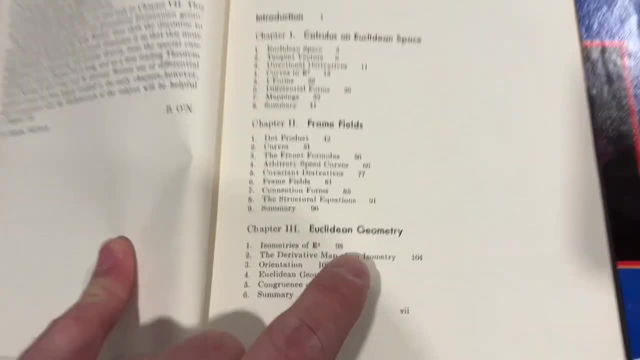 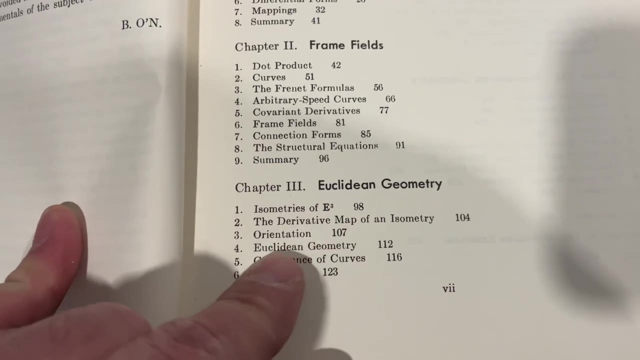 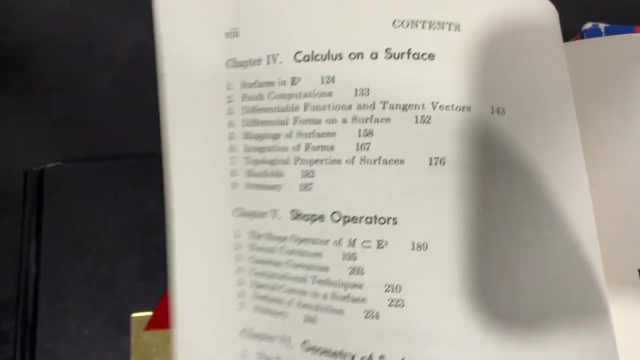 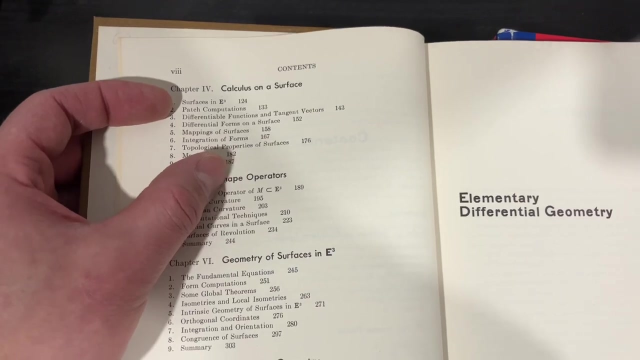 Uh, frame fields, Euclidean geometry. So this is what uh Emilio was asking about. So the derivative orientation, Euclidean geometry. A brief summary down there. Uh, calculus on a surface- Very important topic: Mappings on surfaces, Integration of differential forms, Topological properties of surfaces And shape operators. Geometry of surfaces. 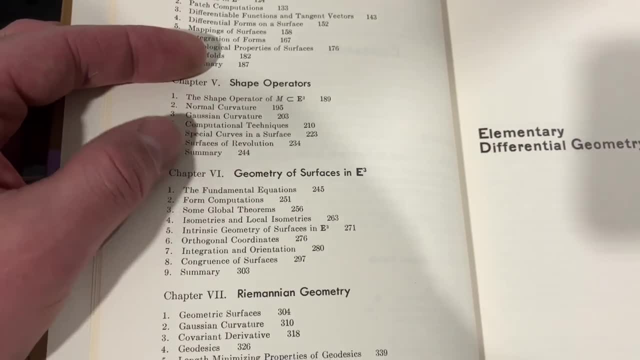 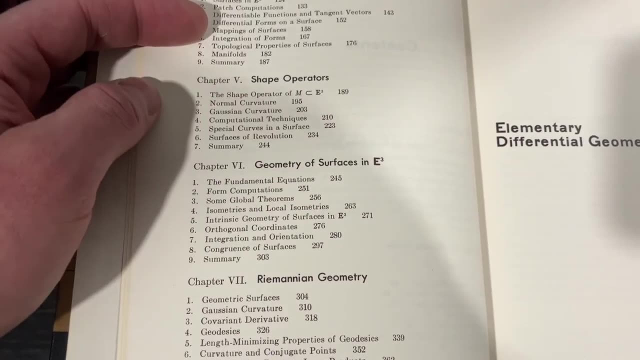 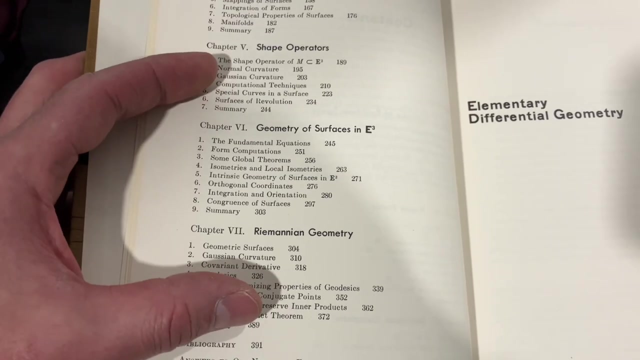 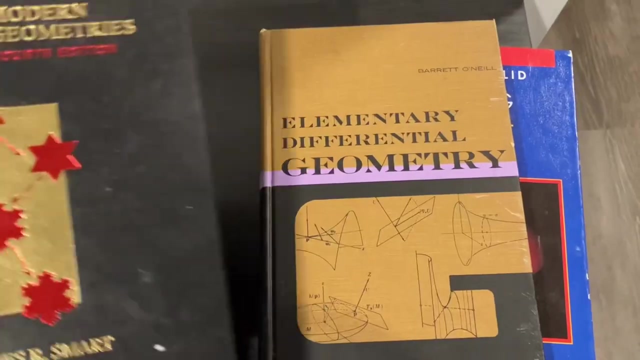 and shape operators. geometry of surfaces in R3- that's an old notation for R3, the Euclidean space. actually E stands for Euclidean, so R3. and then a little bit about Riemannian geometry, so Gaussian curvature, covariant derivative geodesics. it's a very, very nice textbook and this is the, I would say more. 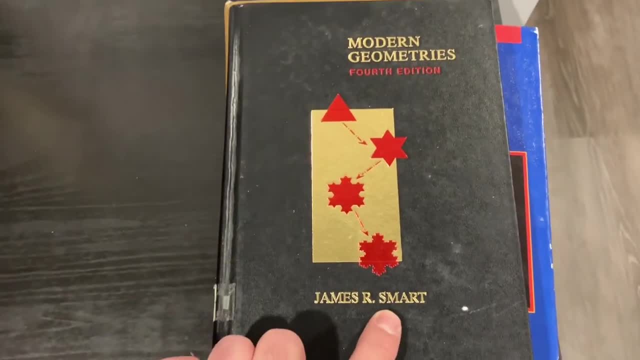 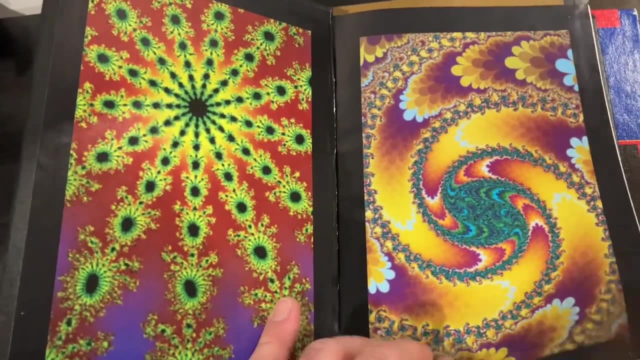 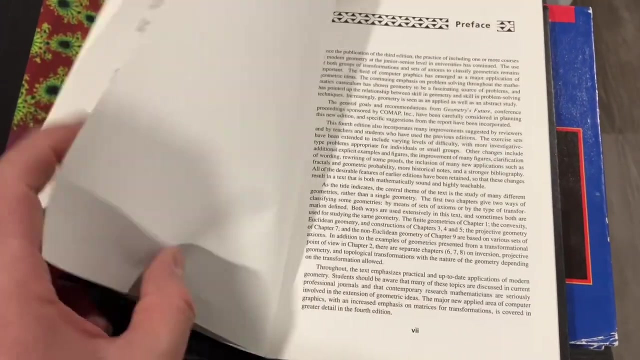 visually beautiful textbook out of the bunch here by smart James: smart, modern geometries. so this is the fourth edition. look at that: some fractal geometry down here. the addition is amazing. this addition is really really beautiful here. the addition is amazing. this addition is really really beautiful. 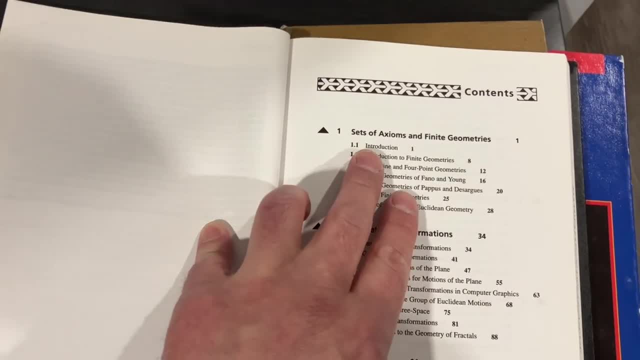 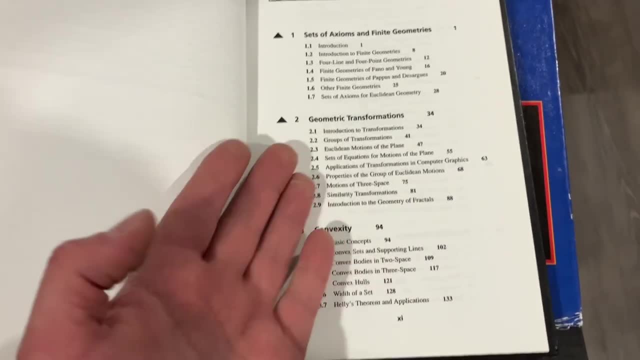 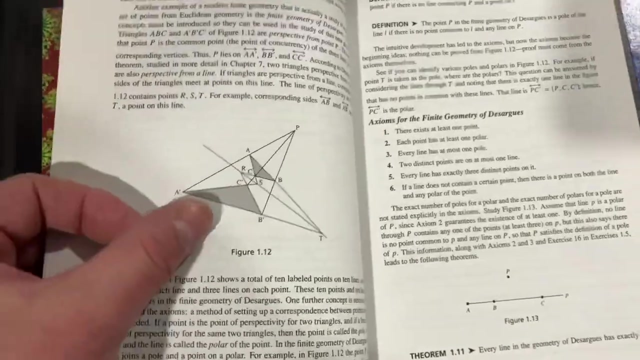 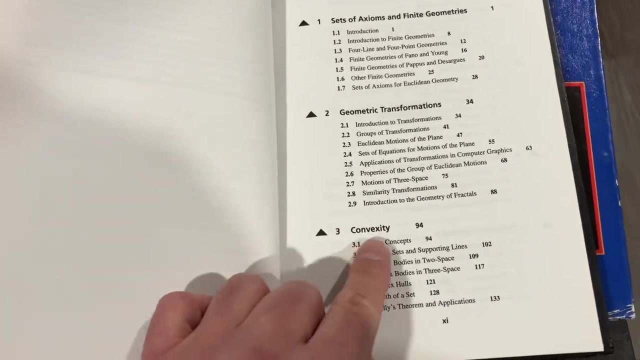 so look at this: axions on finite geometries, four-line and four-point geometries, so groups of transformations. so this is not exactly Euclidean geometry but it's a complement to planar geometry. actually, down here you can take it out: convexity, the notion of convexity, Euclidean geometry of the polygon and 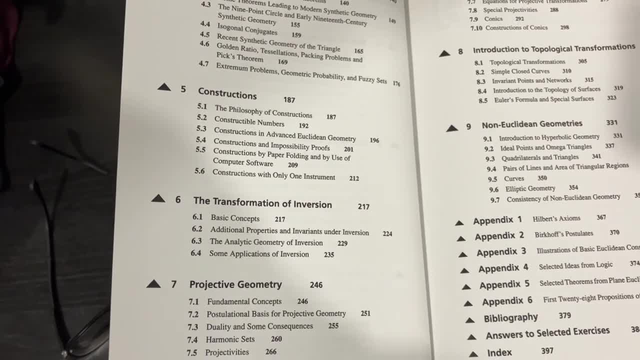 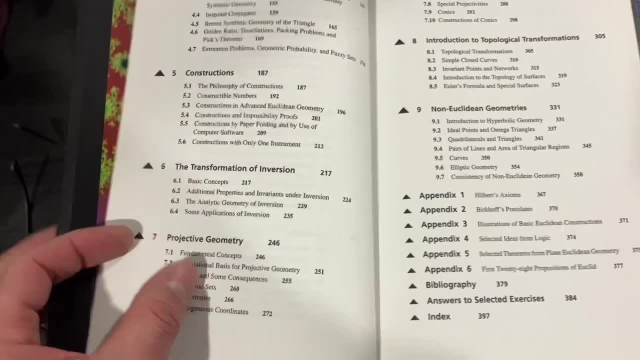 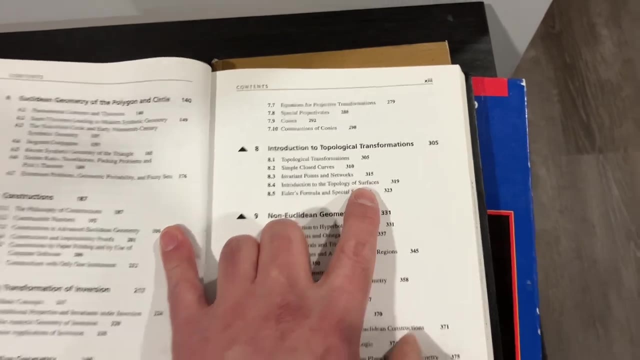 circumference of the polygon and circumference of the polygon and circle, some constructions here. the transformation of inversion in projective geometry- again super interesting and wonderful topic for sure. introduction to topological transformation, introduction to the topology of surfaces, I believe. I do believe they treat, you know the. 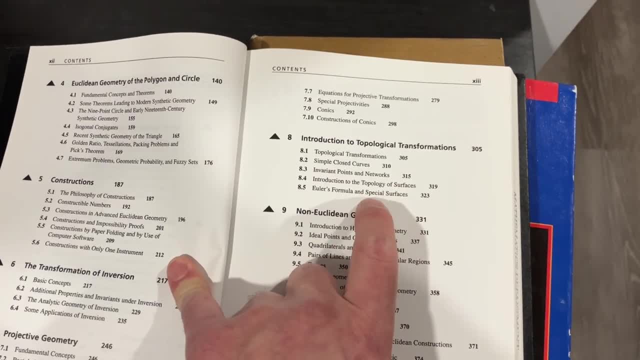 invariance of of a surface. I don't believe they go up to homology groups and stuff like that, but like they don't go up to homology groups and stuff like that. but like they don't go up to homology groups and stuff like that but like they don't. 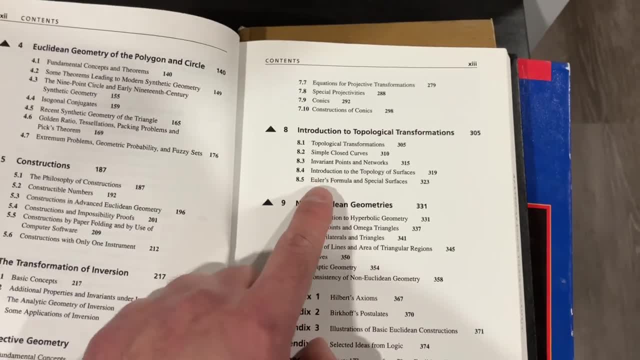 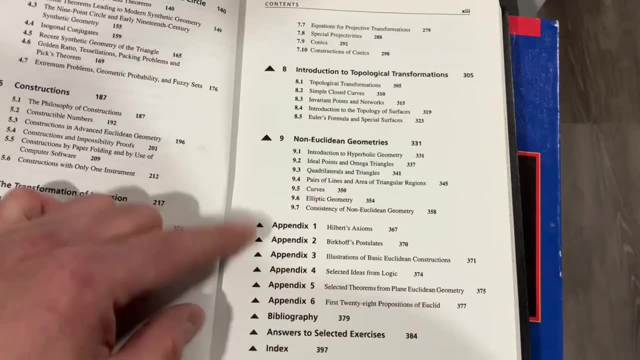 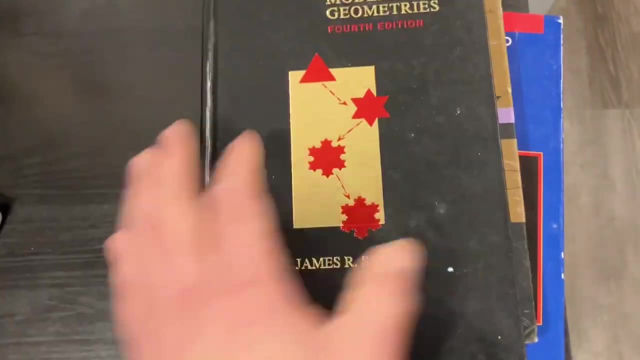 do. yeah, it's right here. they do visit here on earth, entrepreneurs, formula and special surfaces and then some non Euclidean geometries down there. a bunch of appendices so you guys might check it out. you might like to have a look at this wonderful textbook. tons of exercises done. they're insightful. 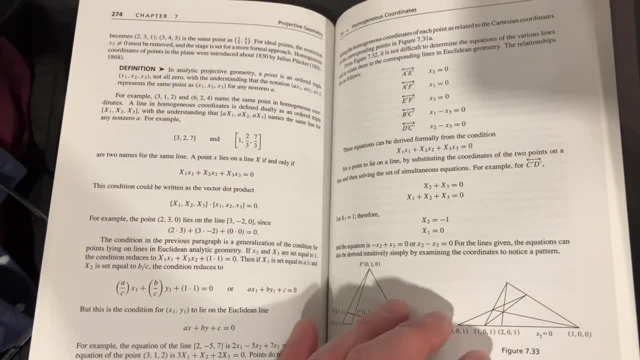 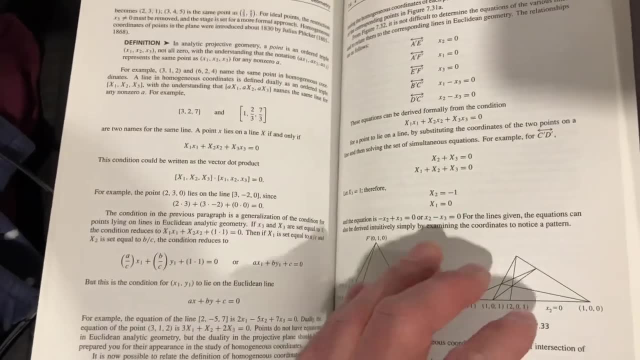 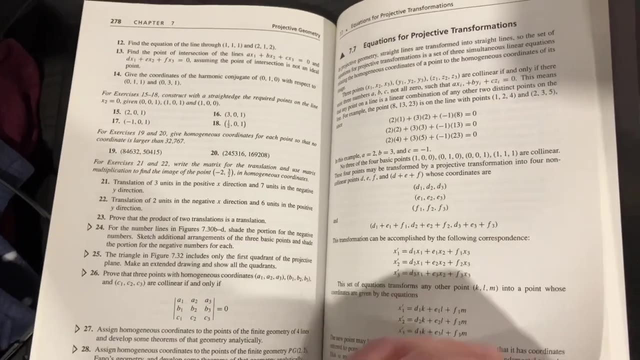 homogeneous coordinates down there. So the homogeneous coordinates are, you know, the coordinates of a projective space actually. Well, it would take another video to talk about projective geometry, but plenty of wonderful examples down here. Equations for projective transformations.